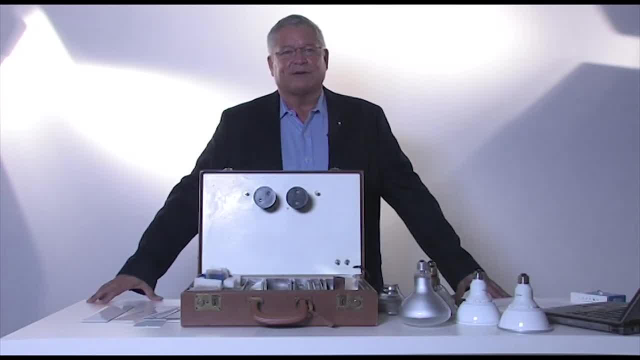 a safe electrical connection to allow for an installation that is appropriate for the architectural details, to enhance the aesthetic or the look and, lastly, to control the light. To control the light, there's really two aspects of controlling the light that optics are concerned with. That is, delivering the light where you want it to go, but also impacting. 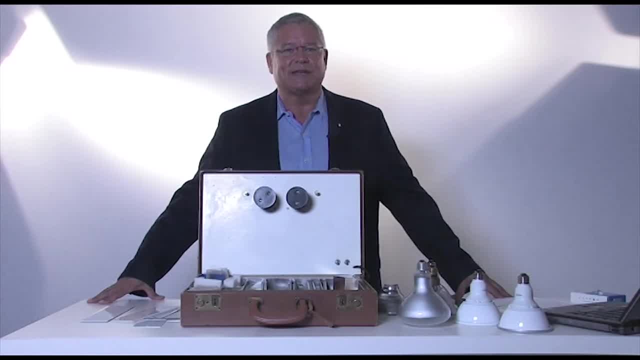 the overall appearance as you look at a lighting instrument That is to control glare and to provide shielding so that we can reduce the brightness and provide for visual comfort. There are two basic physical principles that are important in doing this. They are reflection and refraction. Let's take a look at them. 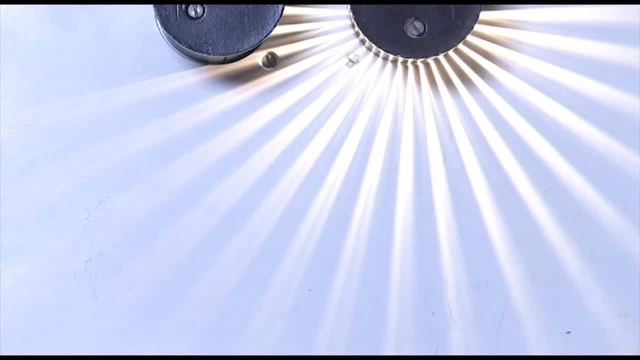 So when we take a look at refraction and reflection, it's important to isolate the component of light into basically an individual ray. I'm going to use this device, which is currently showing you an entire abundance of arrays of light in all directions. I'm going to isolate that basically to one single. 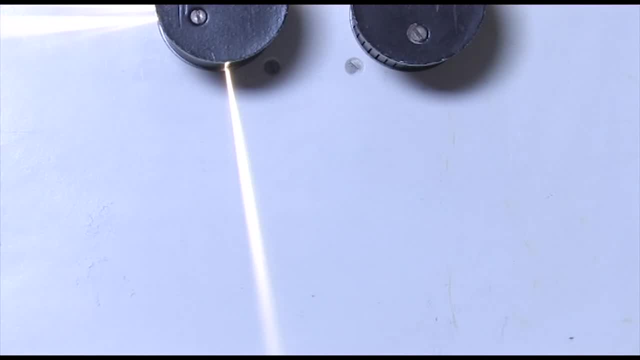 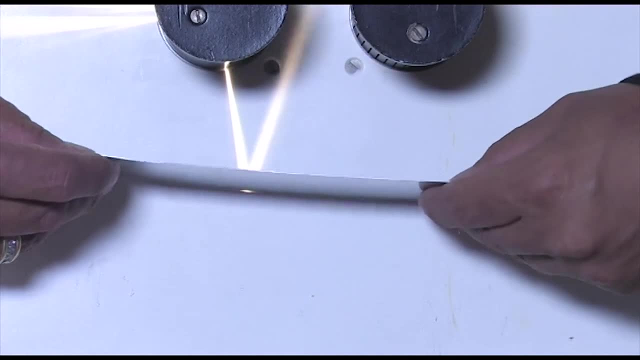 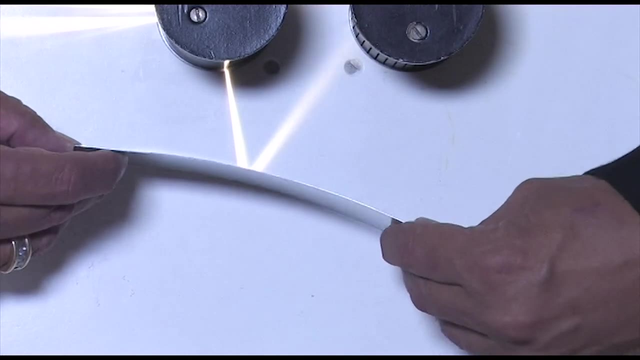 ray, so we can talk about light. Our first physical principle is reflection. The important thing about reflection is that the angle of incidence is equal to the angle of reflectance. Once I understand that principle, all I have to do is to adjust the contour of the reflecting body and I can shape that to actually change the direction. 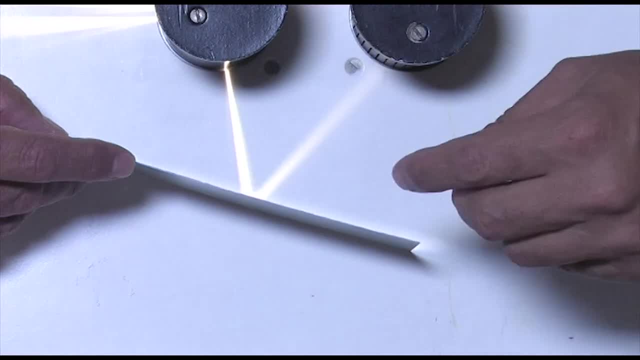 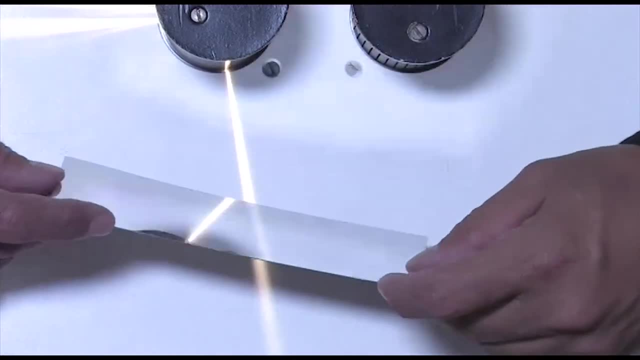 in which light travels. Reflection tells us that the angle of incidence, that is, the angle at which light comes into a surface, is equal to the angle of reflectance when I have a highly polished or specular surface, When I have a more diffused surface, in fact. 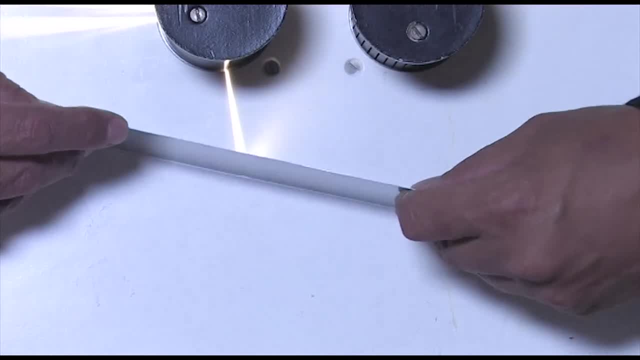 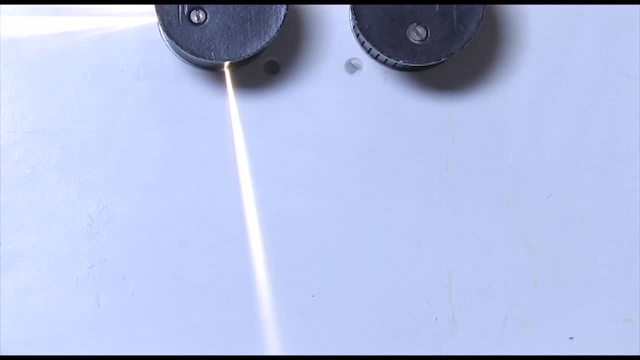 I get less specific reflections off of that surface and much more difficult, therefore, to control. The second principle is refraction. I'm going to use prisms to describe the principle of refraction, And when I take a prism, which is an optical solid of unparalleled surfaces, and introduce 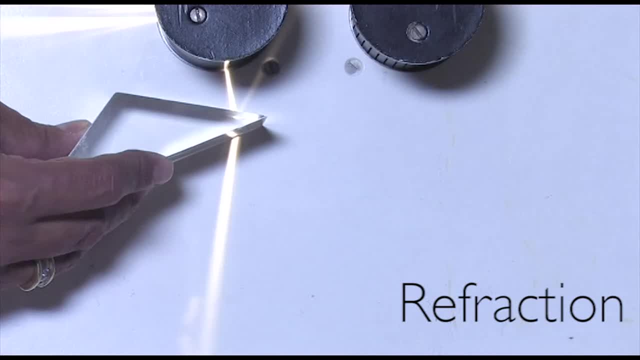 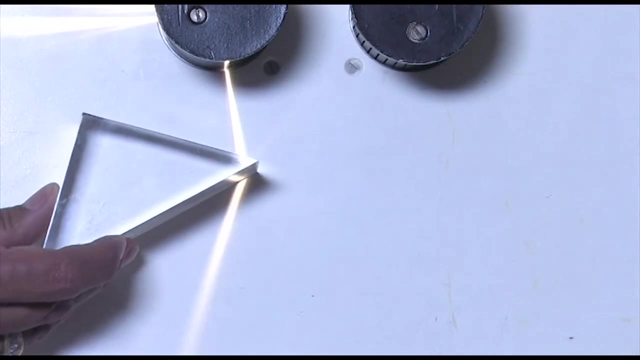 it into the path of the light, well, obviously I bend the path at which light follows. This particular prism is only about 15 degrees, so it doesn't bend the light nearly as much as a prism that is, say, 45 degrees. When I introduce that into the path, it bends the 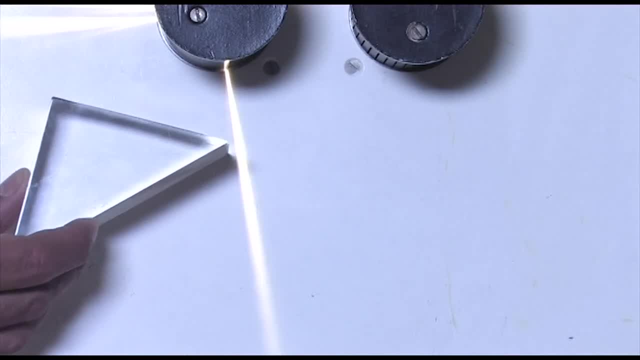 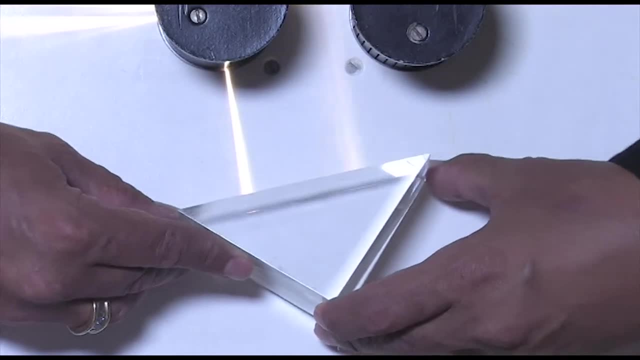 light. even more more Interesting thing about this, although we consider this a refractor, when I have a prism that's 45 degrees, I can also count on it for total internal reflection And in this case, when the light hits the surface at 45 degrees or more, it actually reflects. 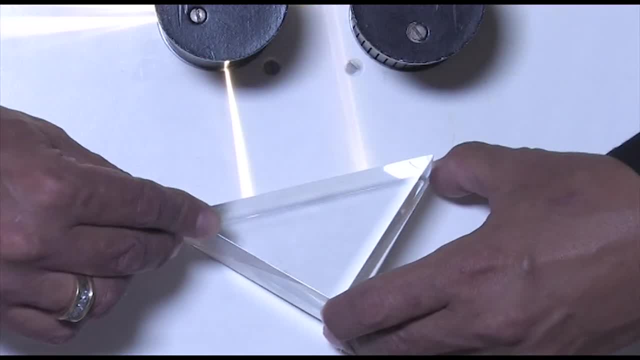 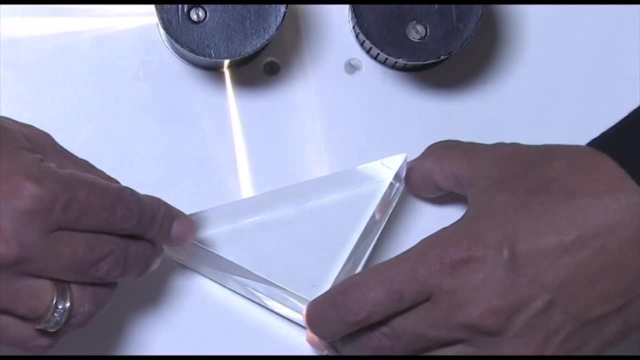 across and reflects back up the other direction, and that is in total internal reflection. This refractor is used in internal reflection property on industrial fixtures, as we'll see in just a moment. So when it comes to reflection, we saw that the contour of the 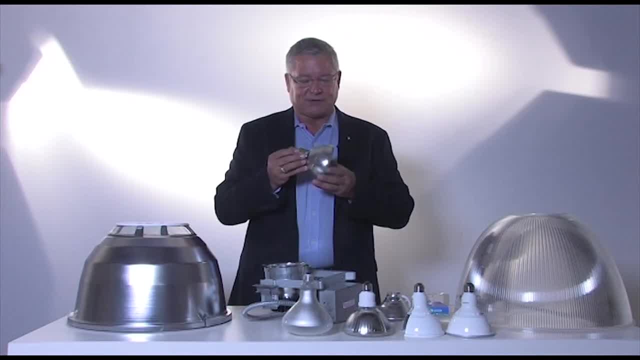 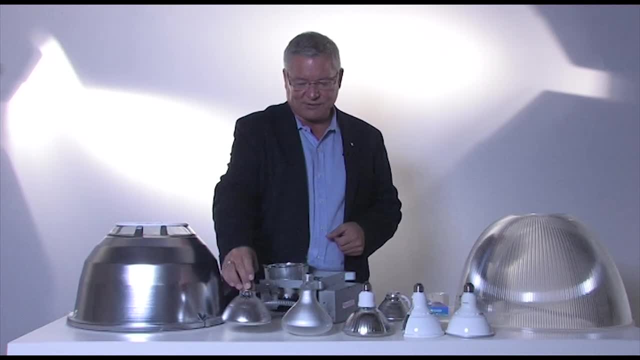 shape is going to impact where light goes, So we talk about a light source. the contour of the shape is going to determine whether that is a spot or a flood source, and whether we're looking for very soft diffused type reflections or whether we're looking for 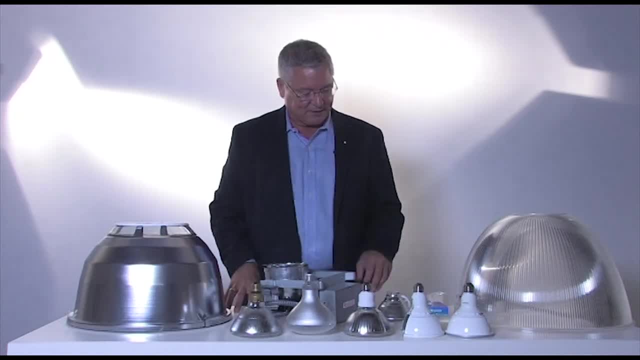 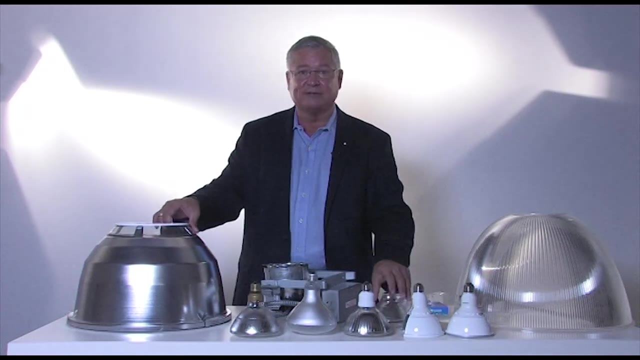 very specific shiny or specular type reflections. When I introduce a light source into that reflector, then I actually start to put into focus exactly where the light needs to go. This is part of the control mechanism. We can do that on a much larger scale, such as with an industrial. 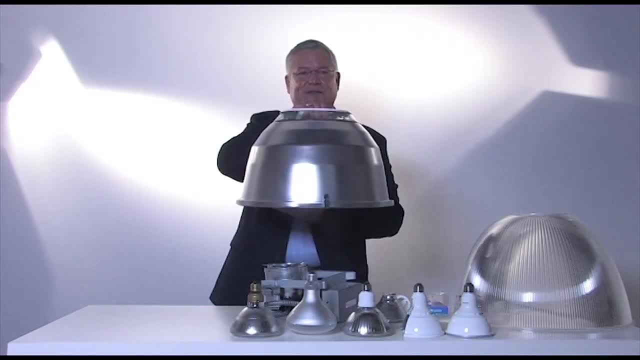 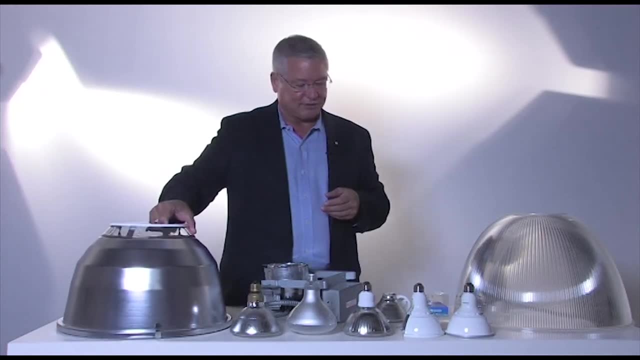 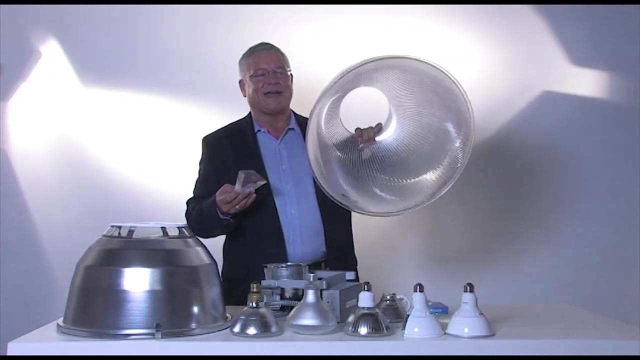 fixture. as we see here And again, the contour of the metal is going to determine what direction the light goes and whether it is specular or diffuse. When we saw refraction, we saw a 45 degree prism being used and the ribs on this particular industrial refractor are. 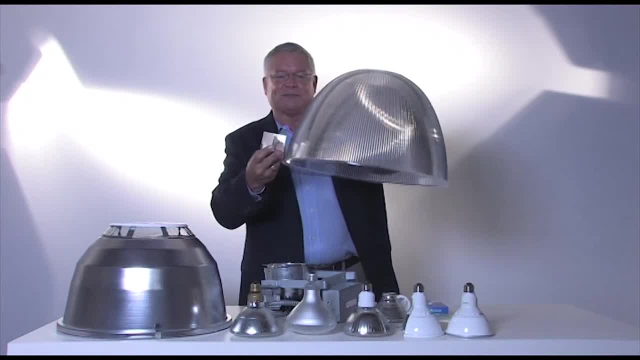 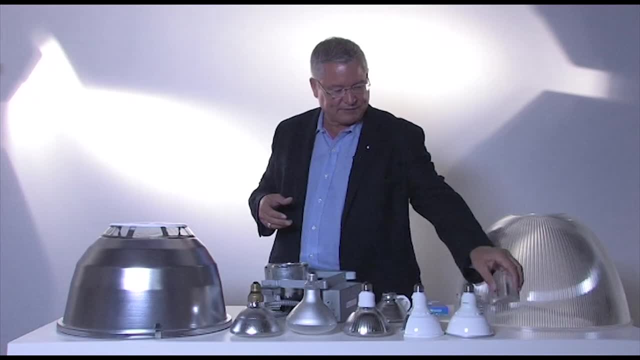 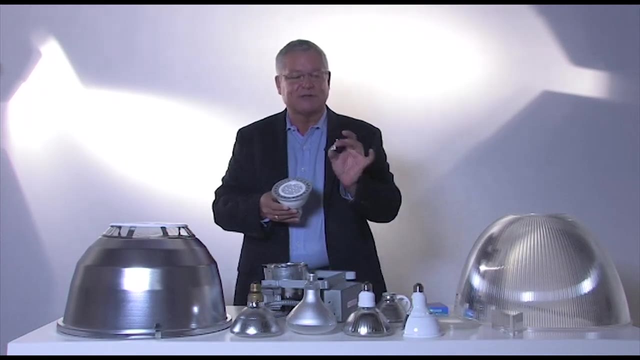 actually just a series of 45 degree prisms that are contoured in shape in order to deliver the light where we want it to go. We do the same thing when we talk about LED sources, although the reflectors that are actually in the source are much smaller devices and actually built into the actual lens of 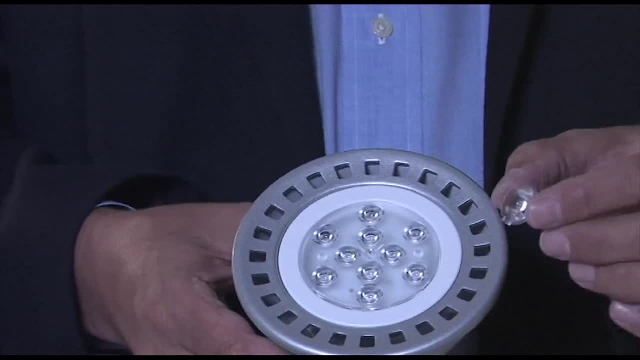 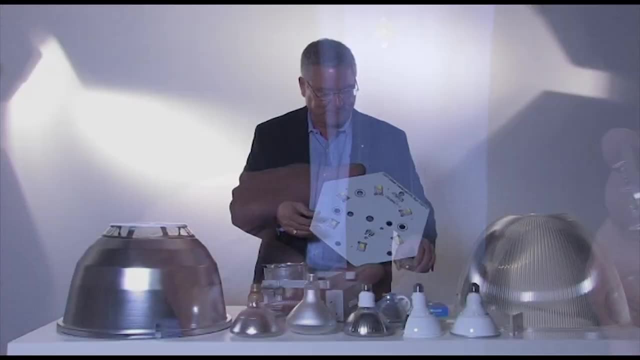 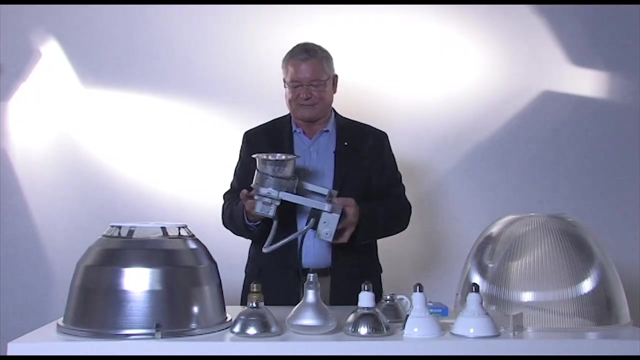 the luminaire itself, such that the reflectors marry and come into focus with the light, making elements to project the light where we want it to go. In a luminaire, be it a downlight, same principles apply. We use a highly specular material for the reflector itself and the